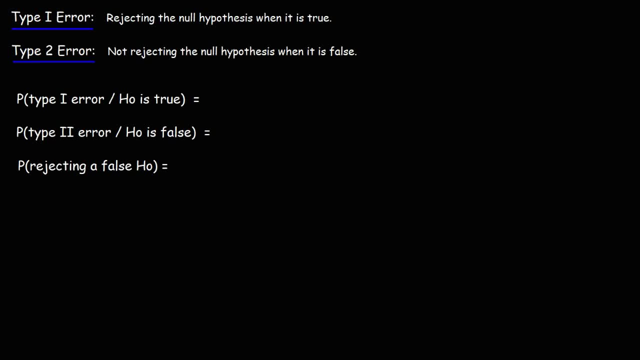 occurs when you fail to reject the null hypothesis when it's false. The probability of making a type 1 error given that the null hypothesis is true- this is alpha. The probability of making a type 2 error when HO is false is beta And the probability of rejecting a false null hypothesis is 1 minus beta, That's. 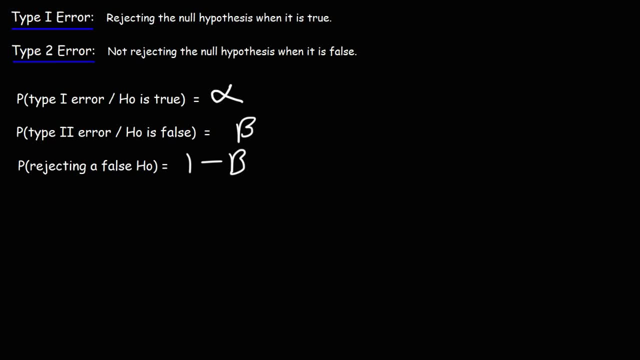 also referred to as the power of the test. Now, what we're going to do is we're going to make a table that's going to summarize all of this. Bear with me one moment. So here we have HO, the null hypothesis, and there's two possibilities: Either HO. 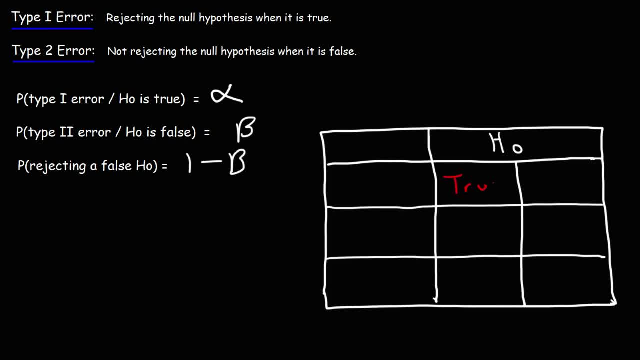 is true or it's false. We can't control that. What we can control is our decisions. We can choose to reject the null hypothesis or we can fail to reject the null hypothesis, which means that we accept it. So those are our two options. So let's say: if the null hypothesis is true and 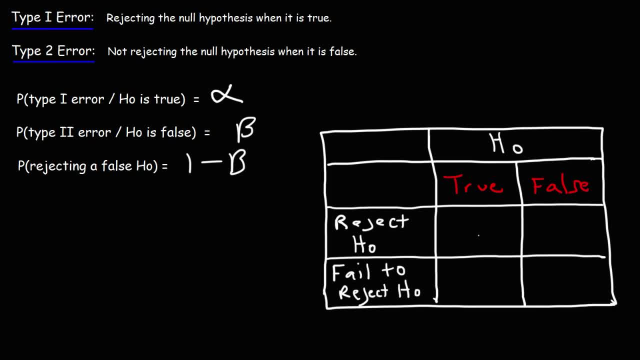 we reject it when it's true, That's an error. Specifically, that is a type 1 error. Now, if the null hypothesis is false and we reject it, then we've made a good decision. That is not an error. Now, if the null hypothesis is true and we fail to reject it or we accept it, that is also a good decision. 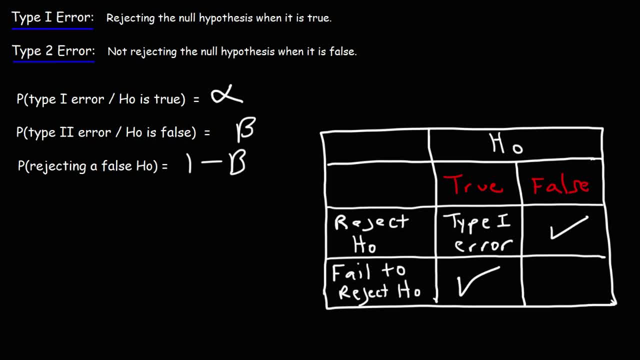 But if the null hypothesis is false and we don't reject it, that's bad. We don't want to accept a false null hypothesis, So that's another error. That is the type 2 error. So hopefully this table helps you to see the difference between a type 1 error and a type 2 error. 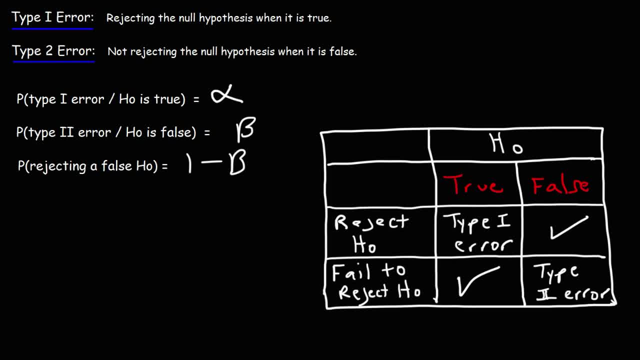 The type 1 error occurs when the null hypothesis is true and we make a bad decision, We reject it. The type 2 error occurs when the null hypothesis is false and we make a bad decision, We don't reject it. Now let's work on the null hypothesis. 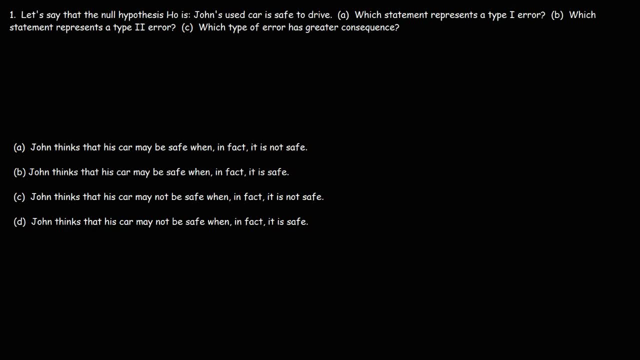 Let's work on some example problems. Number 1. Let's say that the null hypothesis H0, is this statement: John's used car is safe to drive. So that's the null hypothesis, Part A, Which statement represents a type 1 error? 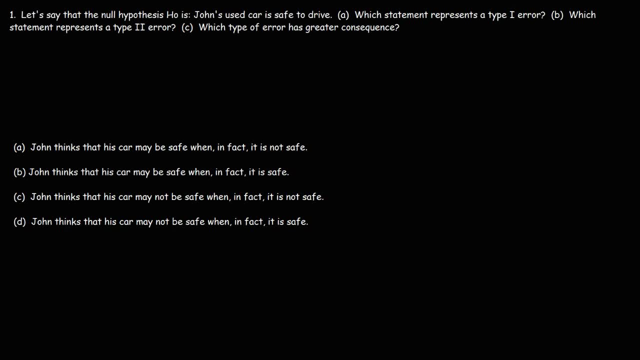 And we could also do Part B simultaneously, Which statement represents a type 2 error. So what I like to do is distinguish the good decision From the bad ones. Let's look at answer choice A first. John thinks that his car may be safe when in fact it is not safe. 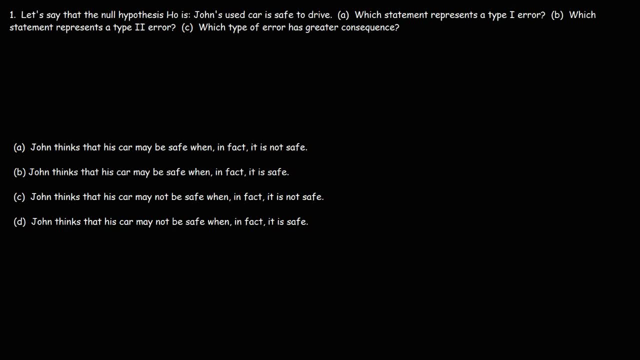 Is that a good decision or a bad decision? Let's say, if he drives his car believing that it's safe when it's really not safe, That's a bad decision. That would be an error. B John thinks that his car may be safe when in fact it is safe. 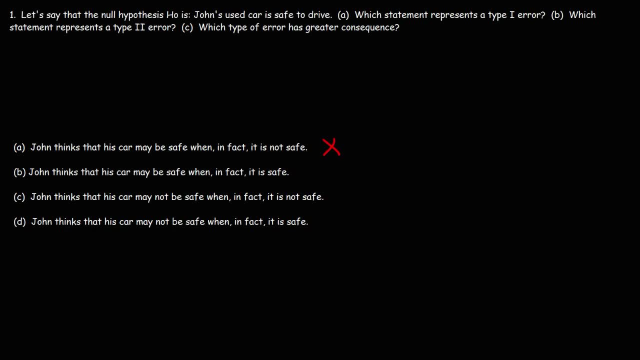 If the car is safe and he decides to drive it, That is not a bad decision. That's a good one. C John thinks that his car may not be safe when in fact it is not safe. So if the car is not safe and he doesn't drive it, that's a good decision. 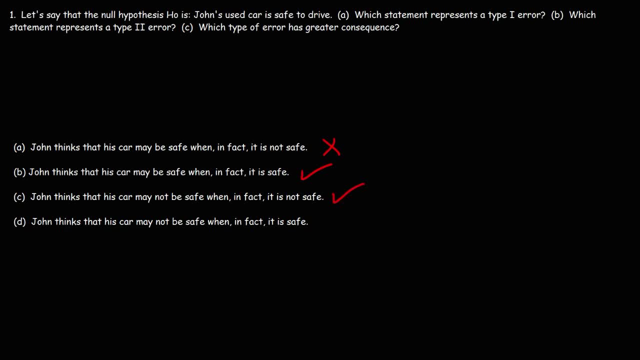 D John thinks that his car may not be safe, when in fact it is safe. That's a bad decision. If the car is good to drive and he doesn't drive it, it that's not really helpful. So that's an error right there. Now we want to identify the type one. 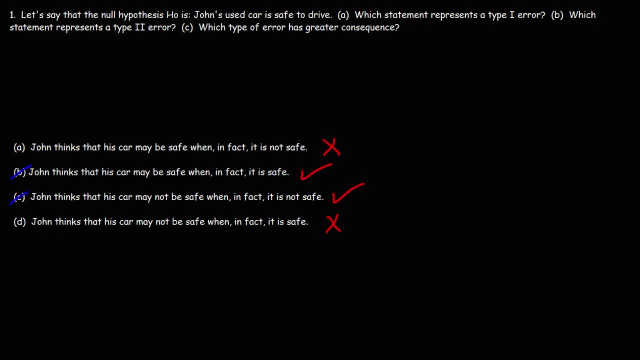 error so we can eliminate answer choice B and C. Now look at that answer, choice A. Would you say it's a type one error or a type two error? Feel free to pause the video and think about it for a moment. Now remember: the type one error occurs when we reject the null hypothesis, when HO is. 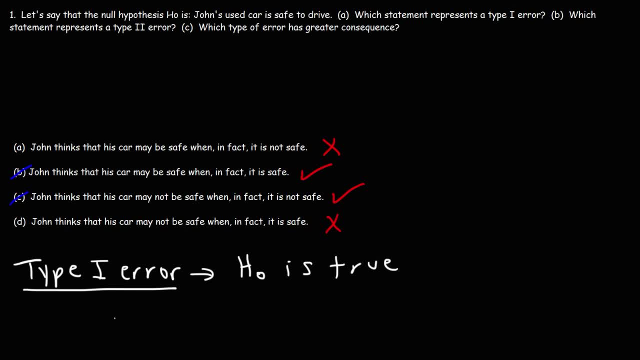 true. It never occurs when HO is false. The type two error. this one occurs when we don't reject the null hypothesis when HO is false. So at this point we need to determine when HO is true and when HO is false. So we know HO is. 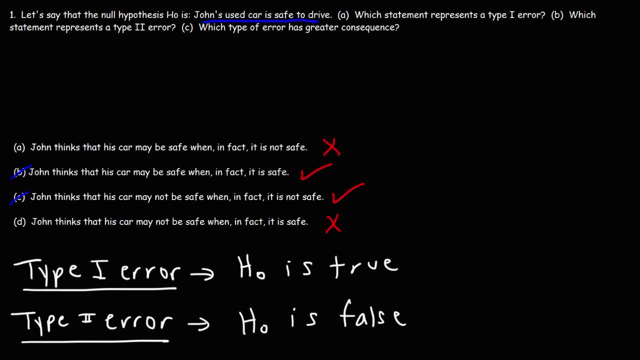 John's used car is safe to drive. Answer choice A is saying that it's not safe to drive. So it's saying that the null hypothesis is false because it doesn't agree with it. So since we have a false HO and he fails to drive, we need to determine when HO is true and when HO is false. 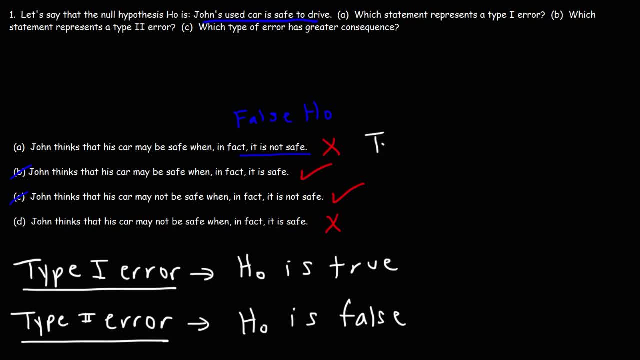 So we need to determine when HO is true and when HO is false. So we need to determine when HO is false. So we need to determine when HO is false. So it's happening now and now. I'm going to reject the false HO. This is a type two error. Now, looking at the 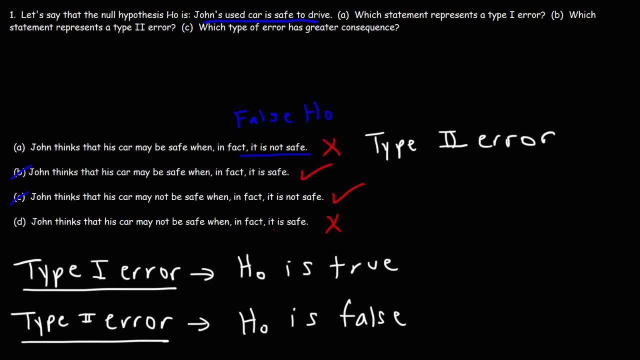 other option, we could see that it agrees with the null hypothesis. the car is safe to drive. However, he doesn't accept it. He rejects the car. He doesn't feel that it's safe. So this is a type one error: He rejects the null hypothesis. 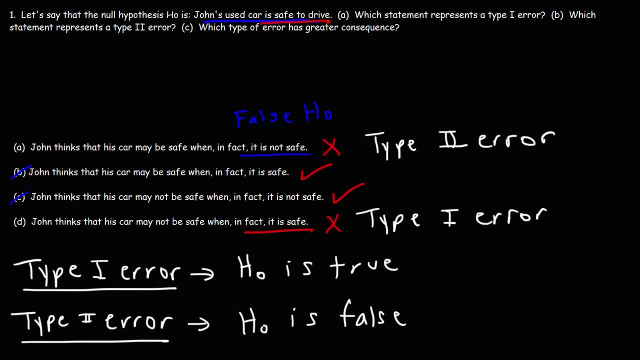 when it is true. So that's a simple way to distinguish a type one error from a type two error. Now let's move on to part C. Which type of error has greater consequence, Would you say it's the type two error or the type one error? Well, let's look at answer choice D first. 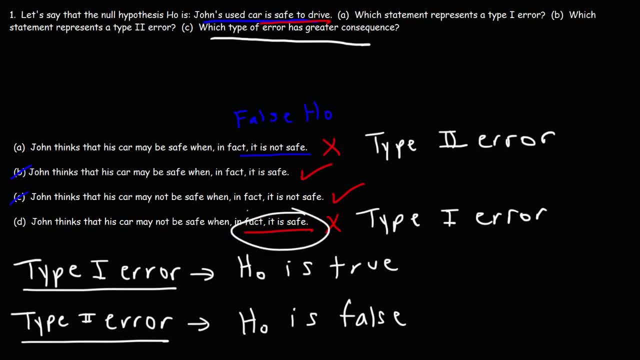 D says the car is safe, but John doesn't believe that it's safe to drive. So if he feels that way, he's probably not going to drive the car. He's probably going to stay at home, eat some pizza, watch TV, and that decision really doesn't have a significant consequence. 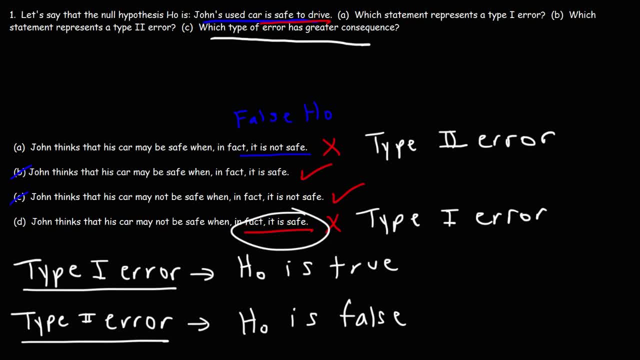 He's going to continue to be alive, so he's not going to get into a car accident. Now looking at the type two error in answer choice A: if the car is not safe, then the car is safe. If the car is not safe, then the car is safe. If the car is not safe, then the car is safe. If the car is not. 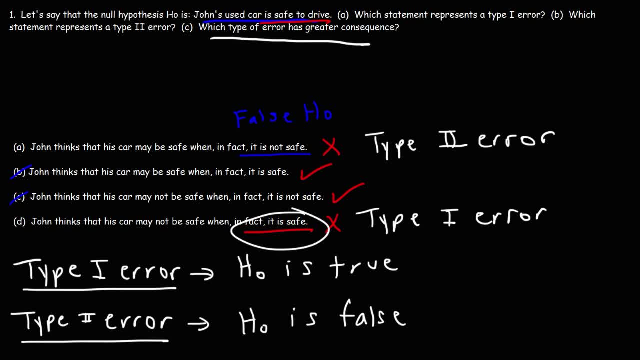 safe to drive. but he believes that it's safe and he goes and drives the vehicle, gets into a car accident, ends up in the hospital. that's pretty bad. I mean he could lose his life. So answer choice A. the type two error has greater consequence Because if he makes that error, 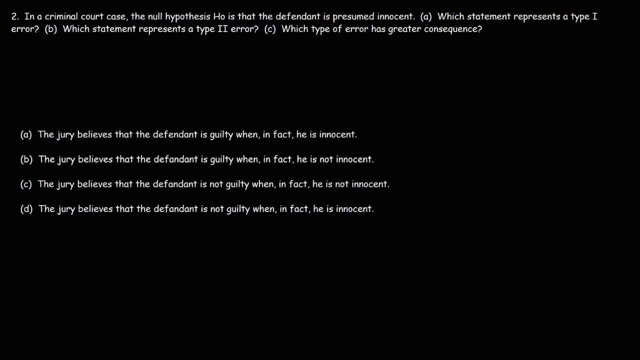 it can cost him big time. It can cost him his life. Now, for the sake of practice, let's work on another example, Number two: In a criminal court case, the null hypothesis HO is that the defendant is presumed innocent. 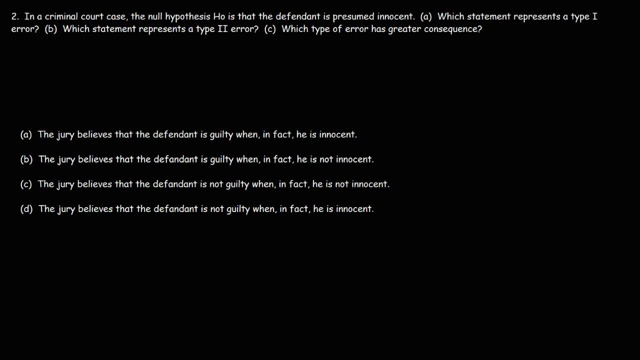 Part A, which statement represents a type one error, And B, which statement represents a type two error. Well, let's distinguish the good decisions from the bad ones. Looking at answer choice A, the jury believes that the defendant is guilty when, in fact, he is innocent. That's not good. So if they pronounce him guilty when he is innocent, 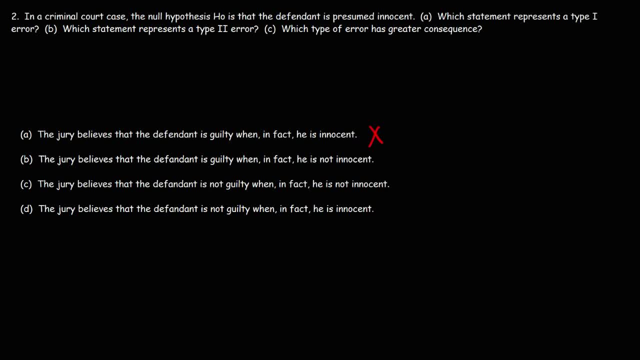 that is a bad decision. That is an error. Part B: the jury believes that the defendant is guilty when in fact, he is not innocent. Okay, that's a good decision. If he's not innocent, he's guilty, So let's put a check for that one. C: the jury believes that the defendant is not guilty. 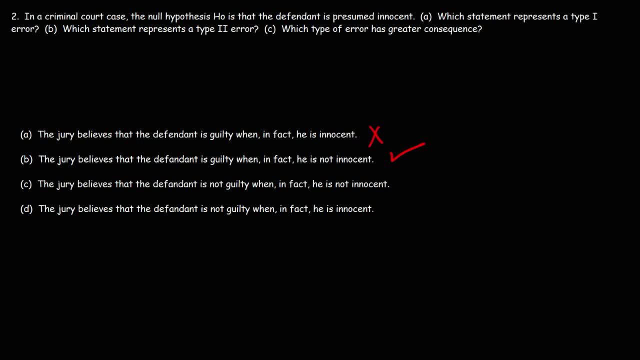 when in fact he is not innocent. If he's not innocent, he's guilty. And if they believe he's not guilty, that is an error. D- the jury believes that the defendant is not guilty when in fact he is innocent. If he's innocent, he's not guilty. So that is a good decision. 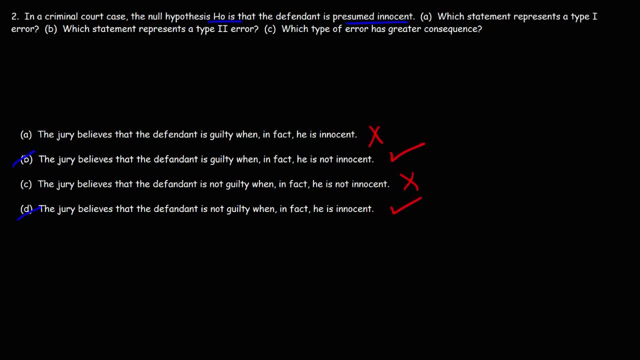 So now let's analyze the two errors that we have. B and D have been eliminated because those two errors are the same. B and D have been eliminated because those two errors are the same. Those are not errors. So let's focus on answer choice A: The jury believes that the defendant